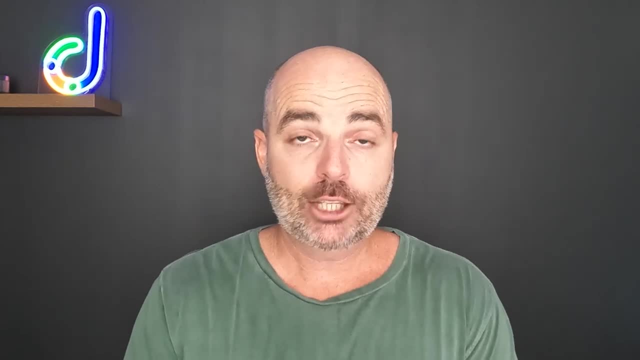 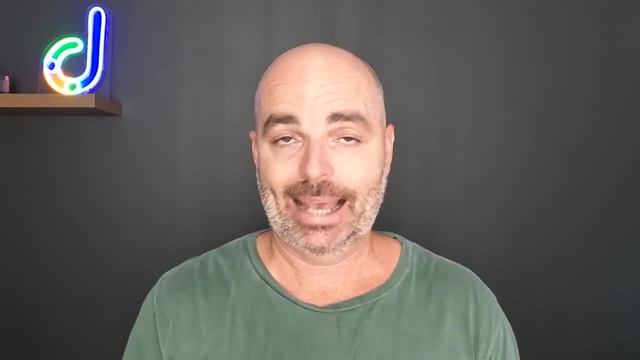 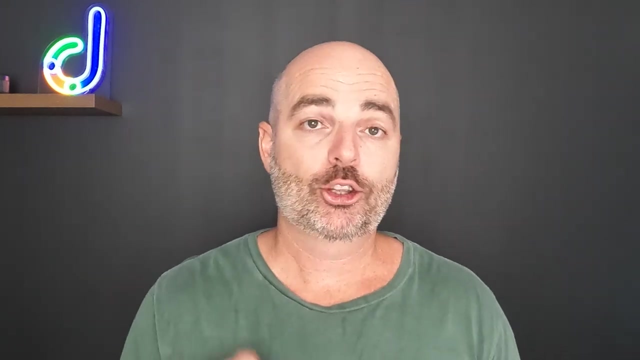 account for a brand that had done no previous marketing. it took us 90 days and seven and a half thousand dollars before we started to see the type of results that we needed to make that campaign profitable. And if you're looking at this video, it's fair to say that you don't have a spare seven or 10 grand lying around to throw into. 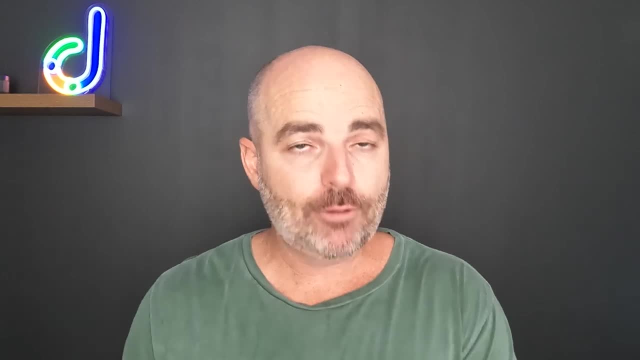 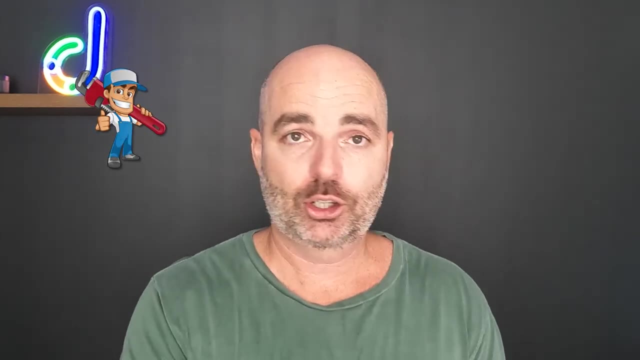 marketing. So that's why I want you to stay away from Performance Max campaigns and focus on search and shopping campaigns. Obviously, if you're a service based business, you would just go with search. If you're an ecommerce brand, I would do a collection, if you can afford it, of search and 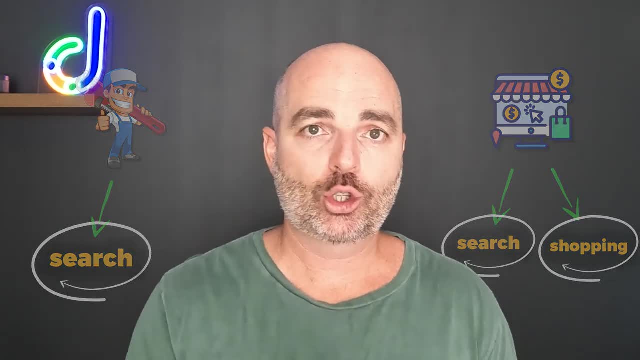 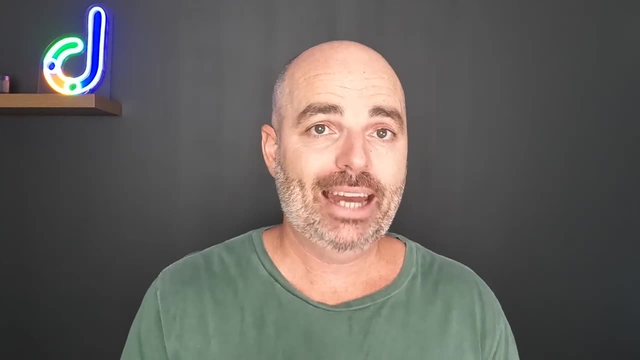 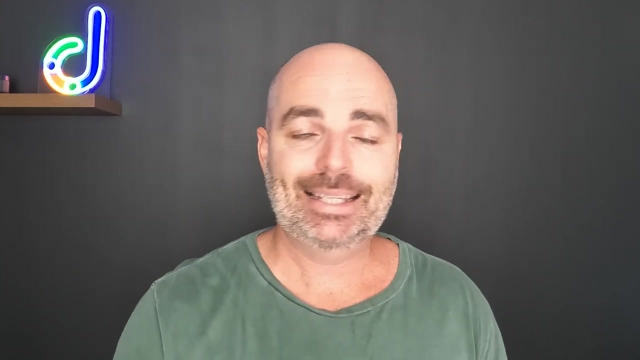 shopping campaigns, And the reason for that is because search ads you can add in some extra elements to your ad copy, especially if you've got some unique selling points which can help get those initial sales across the line. So right now I want to take you through the three core strategies that you can use to still see success. 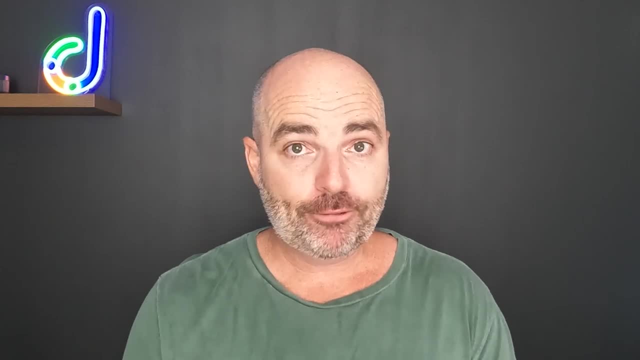 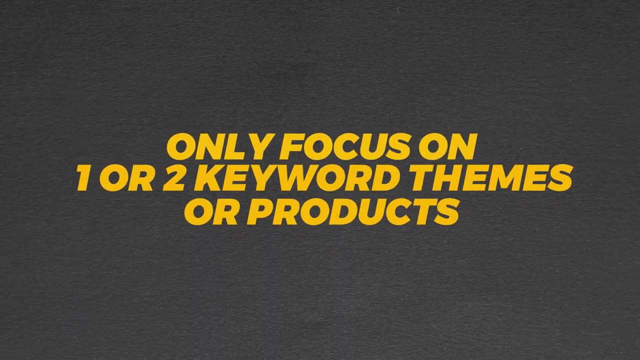 with Google Ads, even if you've only got a small budget, And the first strategy is that when you're starting, I only want you to focus on one or two different keyword themes or products. What the temptation can be is that if you've got multiple keywords and multiple different products, you can 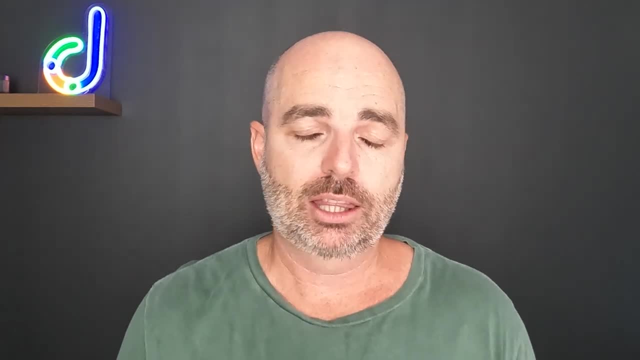 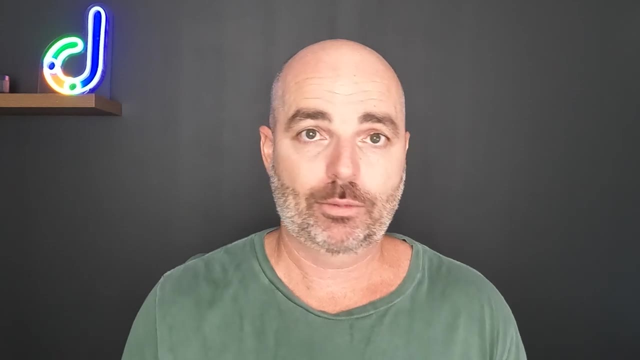 be tempted to market all of those services and products, And the problem is is that you've already got a limited budget. So by trying to market 10 different products or 20 different products or however many different products you've got, there's just too many data points and you 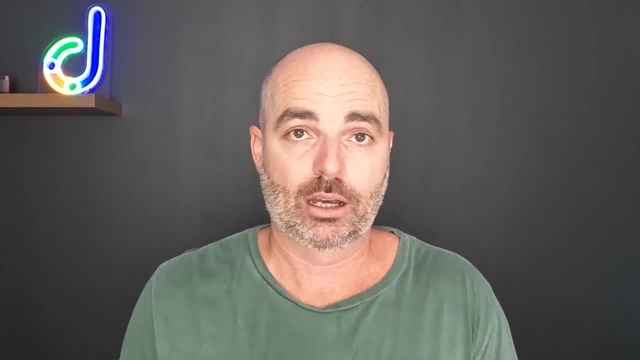 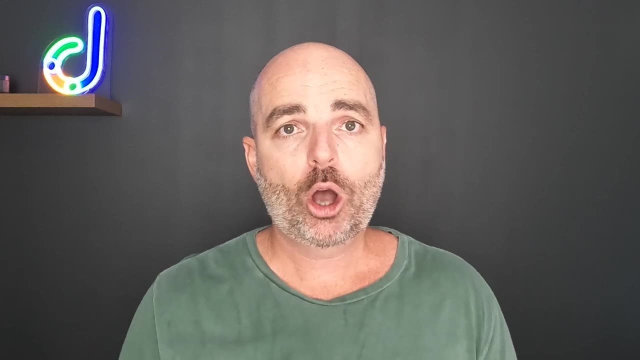 don't have a large enough budget and you're spreading that budget too thin. So, what you want to do and remembering when you're at the start of your Google Ads journey or if you've only got a small budget, what the goal is here is: the goal is to generate some more conversions and some more revenue. so 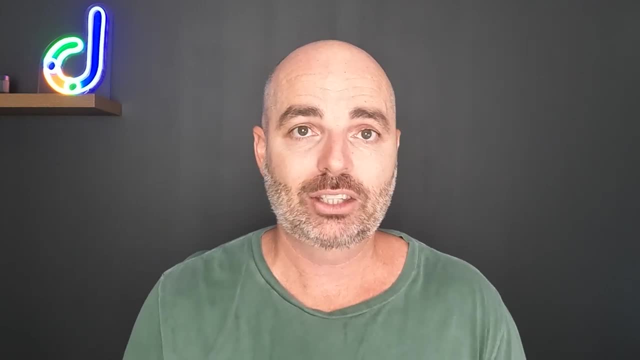 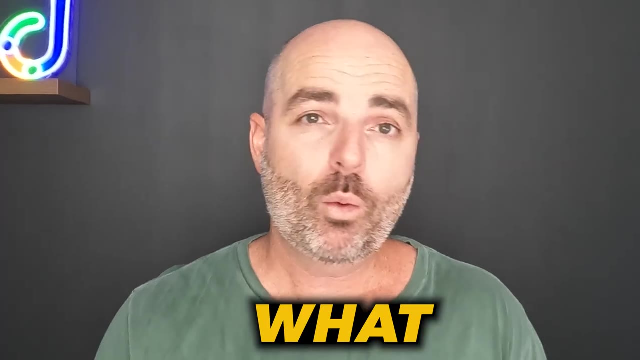 that you can reinvest that back into your business, including your Google Ads campaign, so that you can increase the budgets. So what we're wanting to do here is we're just wanting to focus on what we feel will be the best performing products. Now there's a couple of things that 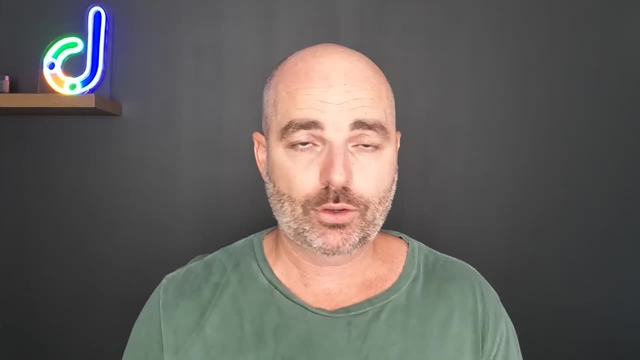 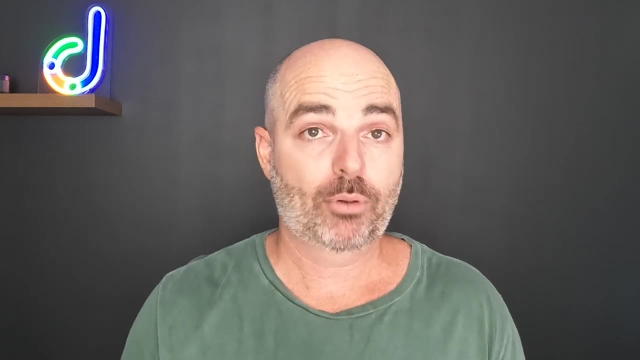 you can do here is that, firstly, you'll know your own products and services, And most business owners would know straight away, or have a really strong feeling on, what are going to be the best performing products at the start, And many of you might term it like going for the lowest. 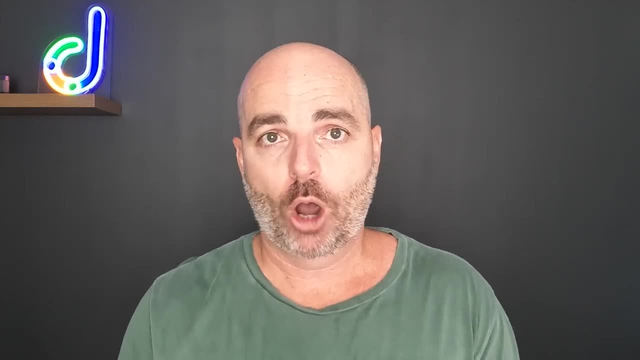 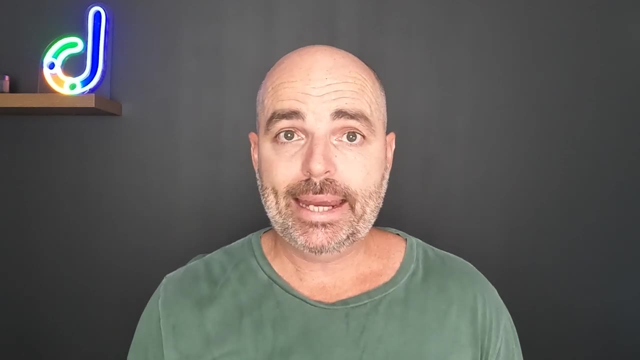 hanging fruit, And that's what we're going for With a low budget. we're going for that low hanging fruit, which we know is going to be the easiest to target and the easiest to convert. So remember. what you wanted to do here is remember because you've got a smaller budget rather than 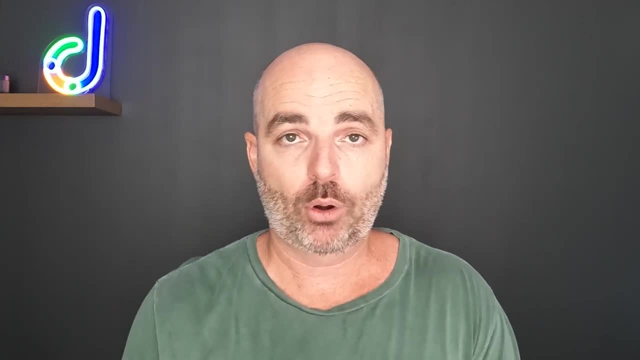 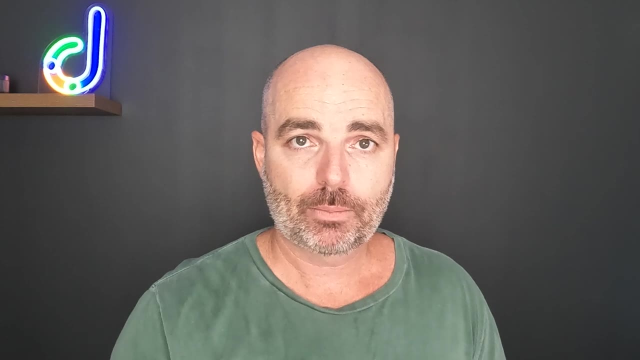 trying to focus on everything you're just looking at, focusing on those one or two products, which is going to allow you to at least be competitive against larger spending competitors in those two areas. Second reason, once again, is because we're going for those more popular products that aren't as 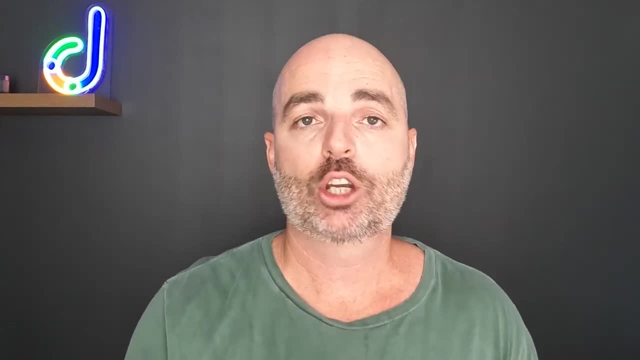 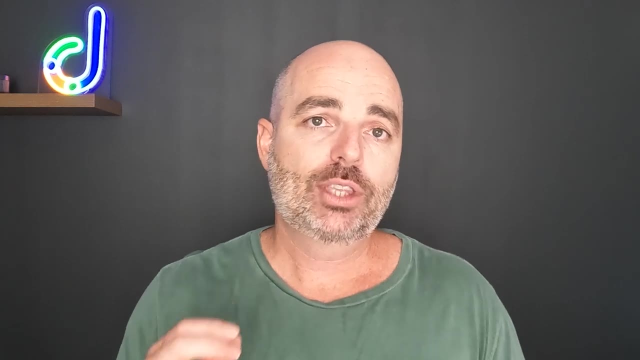 highly targeted, you've got much more chance of success so that you can reinvest that money back into your business. So what I want to do right now is let's jump into a quick screen share, because there is also one other practical step that you can do here, And that is looking at some 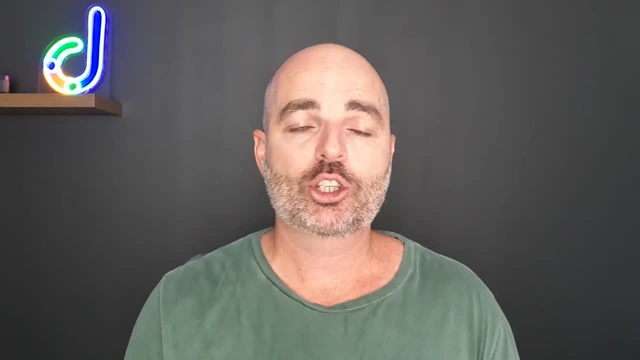 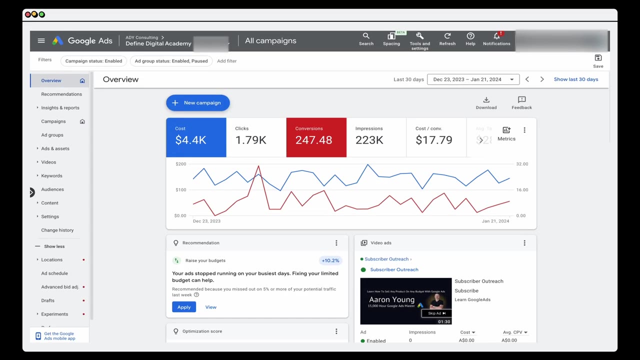 keyword data to find out inside of Google Ads which is going to be the best keywords or the best products to target. So let's jump into that screen share right now. So what we want to do here is we want to go straight up into our tools and settings and go into the keyword planner. If 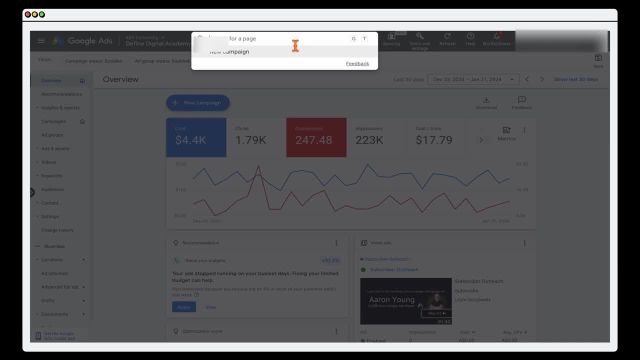 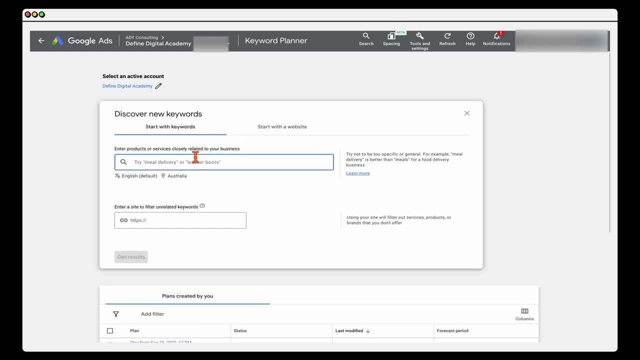 you've got a different version of your Google Ads dashboard. just go into the search bar and type in keyword planner. you can see it's come in here And you want to go to discover new keywords. And what we want to do here is we want to look at the keyword data so we can find the different search. 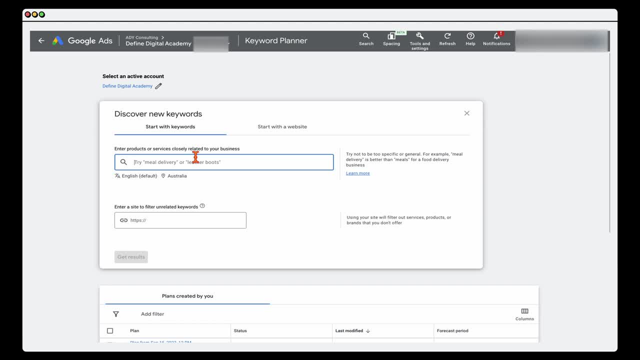 volumes and also the cost of the traffic. So I'm going to run two examples. First of all, we're going to run an example for a local trade business, so an electrician, and then we'll also run an example for an e-commerce brand. So for this one, let's just say that you do air condition. 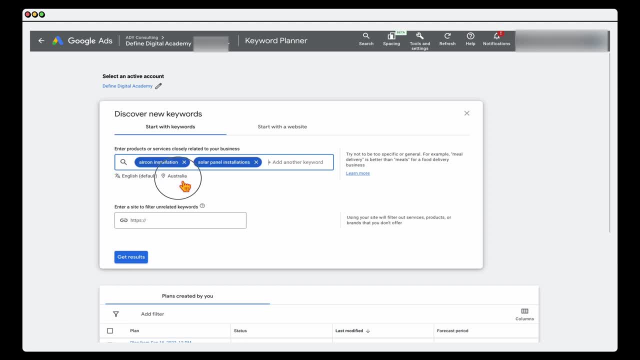 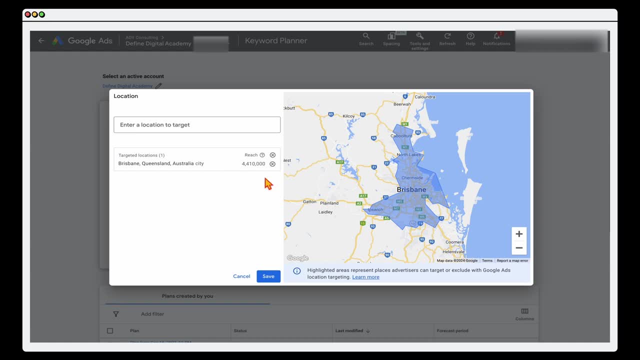 installations and you also do solar panel installations. And I'm going to refine this down to Brisbane only, And that would be another recommendation as well- is, you can also target smaller locations. So I've put in all of Brisbane, but if I wanted to, I could even just go for, say, 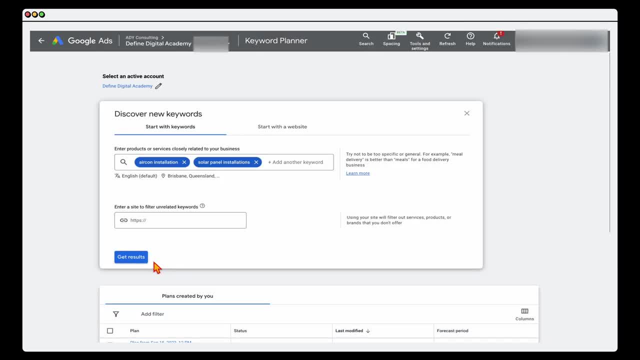 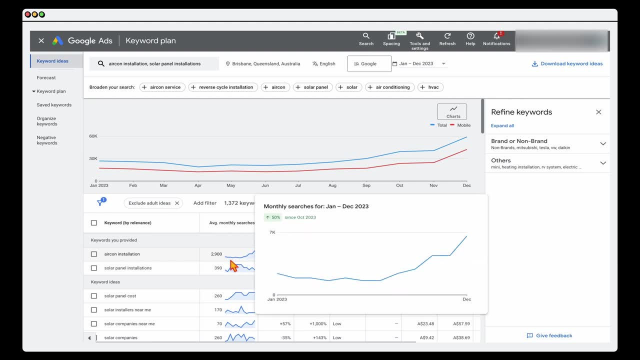 like Chermside and North Lakes, and look at more specific areas, And then, once you've got that, you go through and click get results. So what we're wanting to do here is that we're wanting to look at some data, And the main data we want to look at is obviously the average. 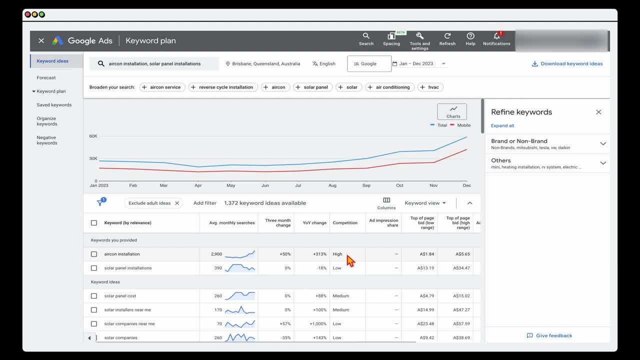 monthly searches. We're wanting to see the competition. Now the competition is just a three point scale, so low, medium or high, And that really lets us know how many other people are competing for these same terms. And then the big thing is: you want to know how much this? 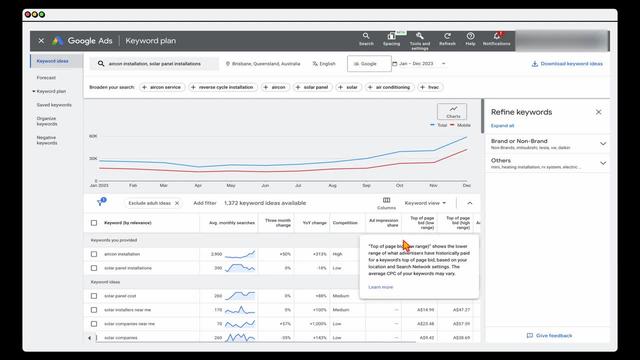 traffic is going to cost you. Now, the difference between this, this top of page bid low range- this would be for your positions three and four, and the top of bid high range is for your first two positions. Now, the other thing that I'd like to say here as well, is that when 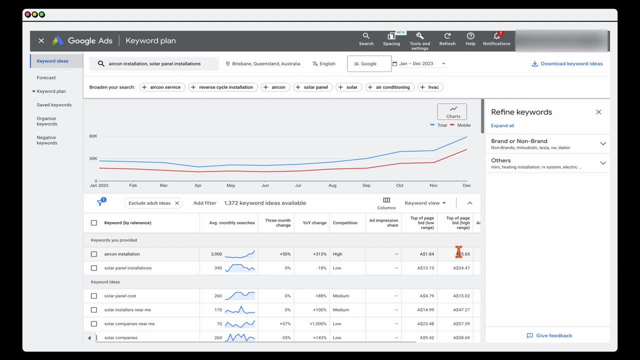 you do set your budgets is that it is important to note that you'd want to be getting at least 10 clicks per day. Now, the reason for why I find that really, really important is so that you've got enough data to optimize your account. So what you need to do is, when you're looking at 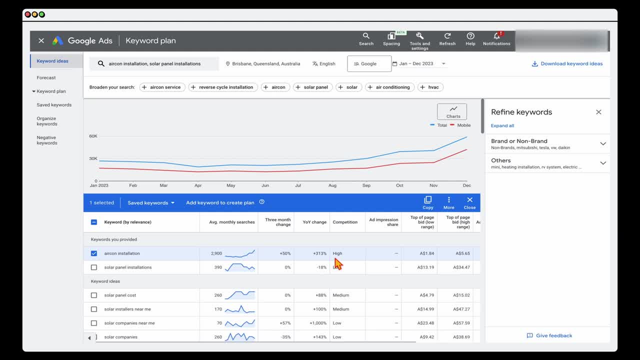 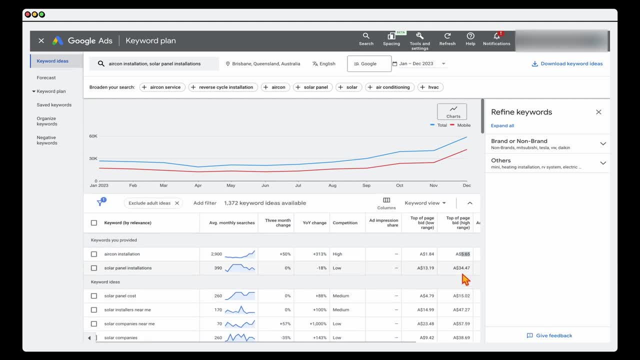 this data here is that you know if you're going to choose air con installation, you'd be looking at the. you'd be wanting at least a budget of $50 a day so that we can get 10 clicks, whereas solar panels that's gonna be more expensive. that would be 340.. So if we know we've only got a maximum of, 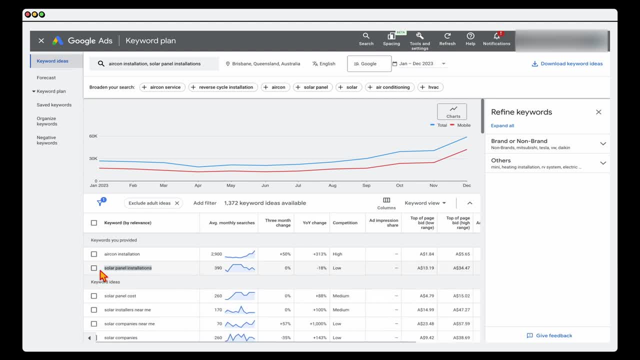 $50 a day. we know straight away that we can't target solar panel installations, And then what you do is you just go down and have a look just to see if there's anything extra that you want to be targeting. So what I would do here is: now that we know that we can't target solar panel installation, 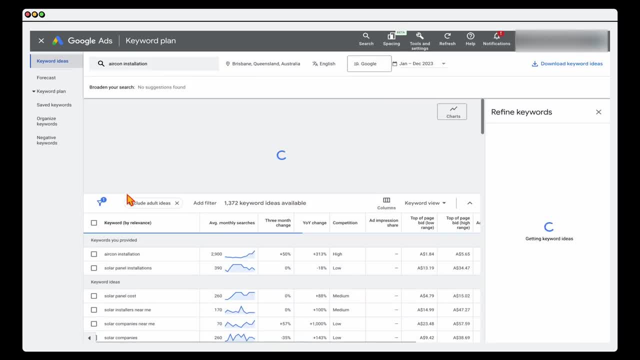 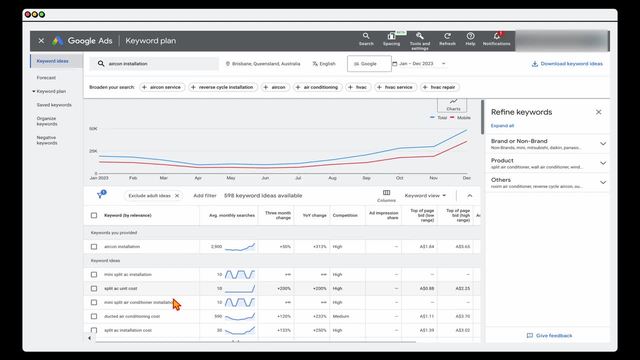 just because the CPC is too high. let's just go air con installation And what we want to look at through here is we want to look at: are there any different variations that we can really target on which is going to be helping us? So you can see here, like with a split AC installation you can 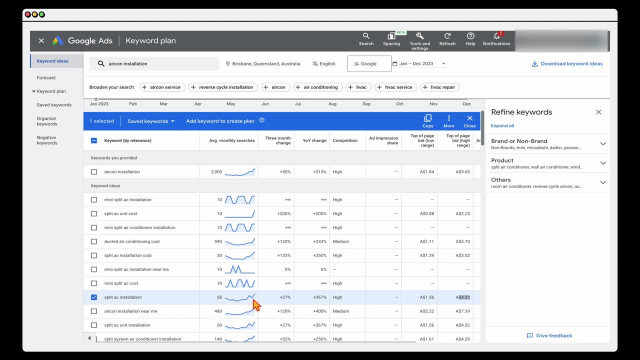 see that the cost per click is just slightly lower And also, as well, there's not as many search terms which, if you've got a lower budget, you're going to be able to target solar panel installation. I tend to stay away from these really high volume keywords. I more look to look at some of these. 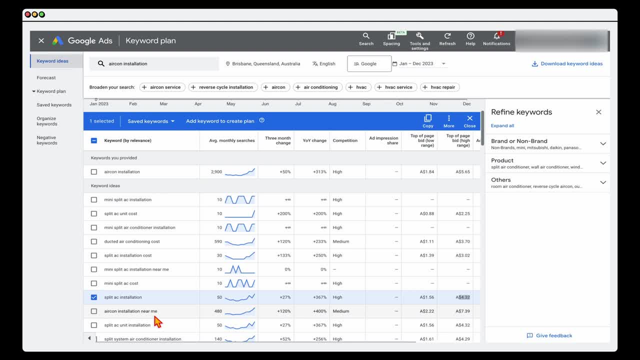 longer tail keywords, because you can generally get a much better return for your business. So I'd be going through these. So split AC unit installation and split AC installation. you can see that we've got that top of page bid down to $4.32, as opposed to $5.65.. 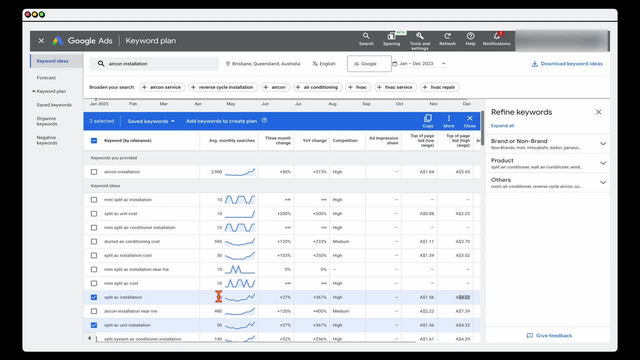 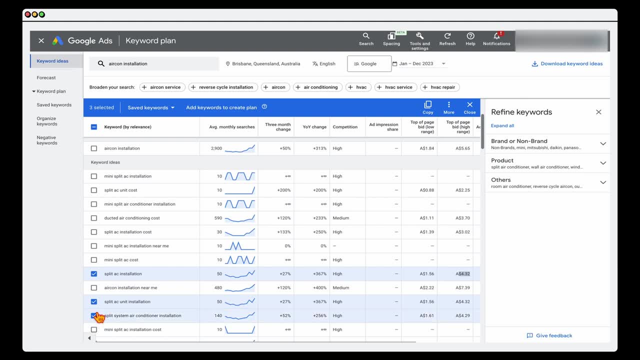 And once again- but we're still looking at this- we've got 100 searches, So that's going to be more than enough for us to be able to target. you can even also add in this one in here Very, very quickly. through that process we've gone from the two products that we highlighted. 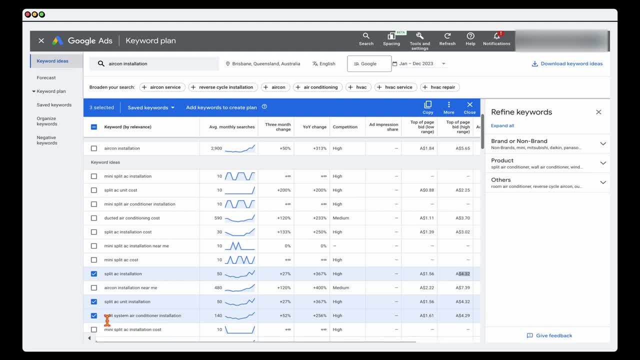 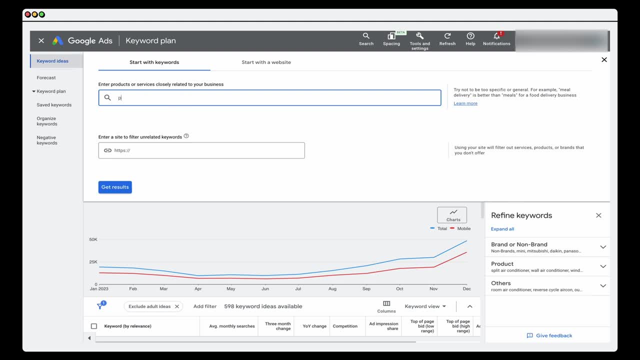 air conditioning installation and solar panel installation. Because of our budget limitations, we've gone. better for us to target on the air conditioning And I just want to show you another example. Let's just say, for an e-commerce brand that's selling gym supplements, we go protein. 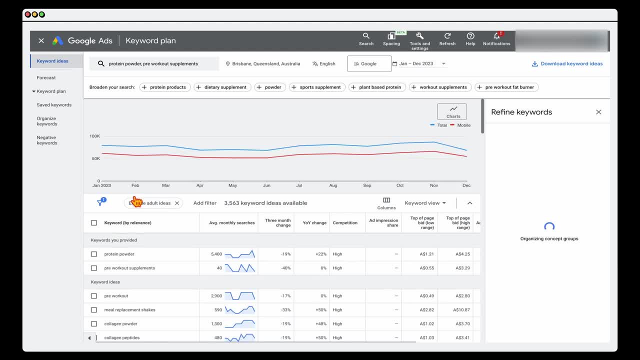 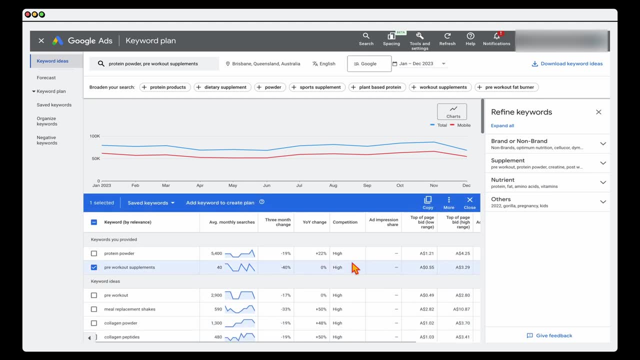 powder and we've gone for also pre-workout supplements. Once again, we want to put that same rationale behind, remembering that we need to be generating at least 10 clicks per day. You can see here that we're going to get cheaper traffic on pre-workout supplements: it's nearly $1 cheaper. 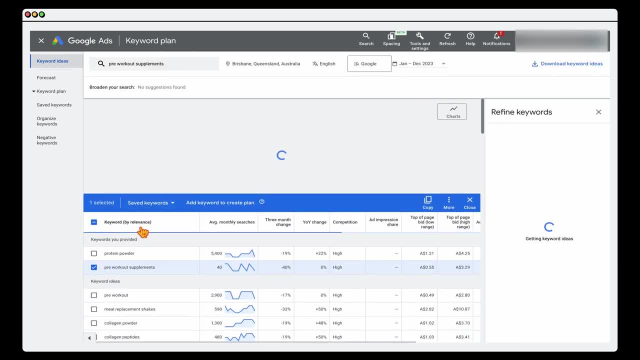 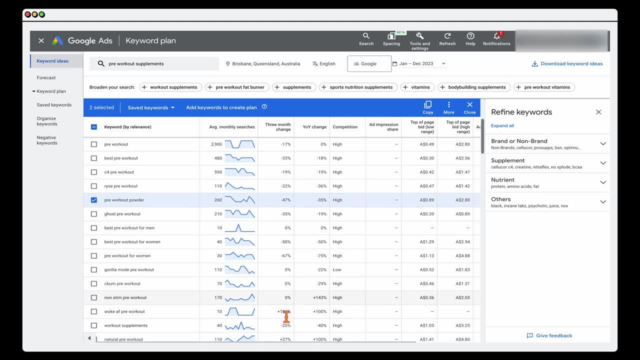 If we then go up and we just say we're just going to focus on pre-workout, What you can see through here is you can then start to go through once again, build out and look to see which are the best search terms to focus on, And what you can even do in here is let's just say there's some. 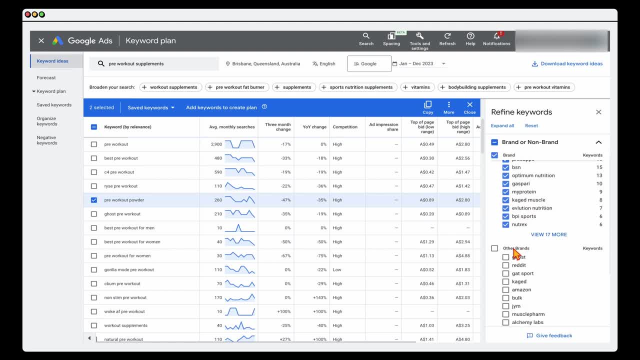 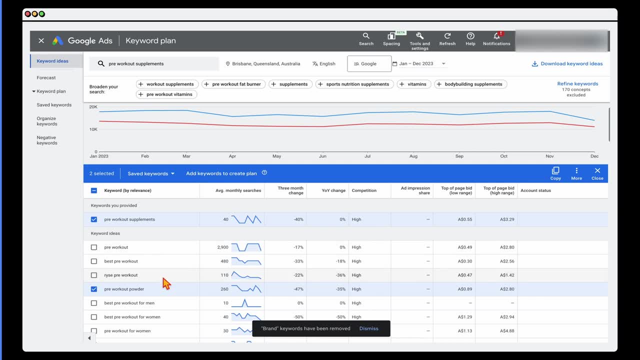 different brands that we don't stock or we don't want to go for is what you can do. you can take these ones out, And we're just wanting to focus on non-brands, And this just gives us a little bit some other data that we can focus on. So remember that first step is looking at focusing on the 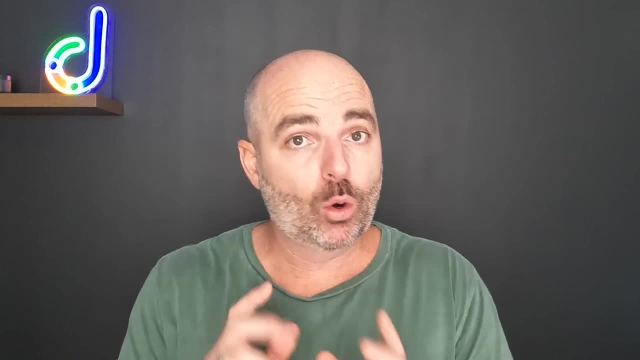 areas where you know you're going to get some good levels of results. So that's what we're going to focus on. We're going to focus on the areas where you know you're going to get some good levels of success And also remembering that key point, that you want to be choosing a keyword theme. 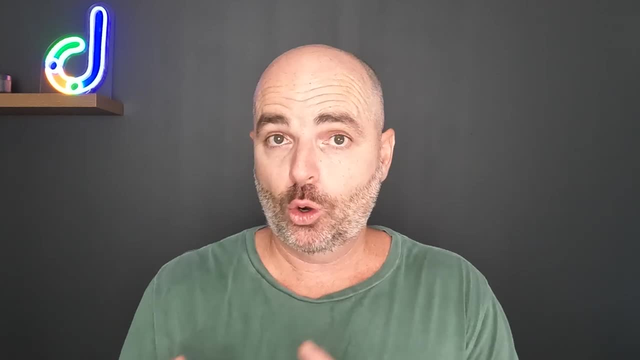 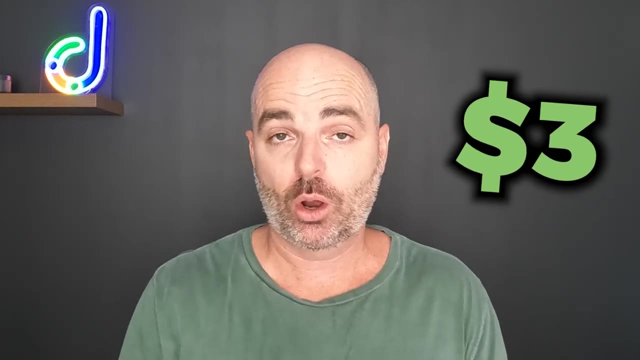 that you can at least get 10 clicks a day from. So make sure you're also reviewing the average cost per click, because if your budget isn't enough for 10 clicks- so if your cost per click is at $3, you would need to be having a budget of at least $30 a day. So that's that two step. 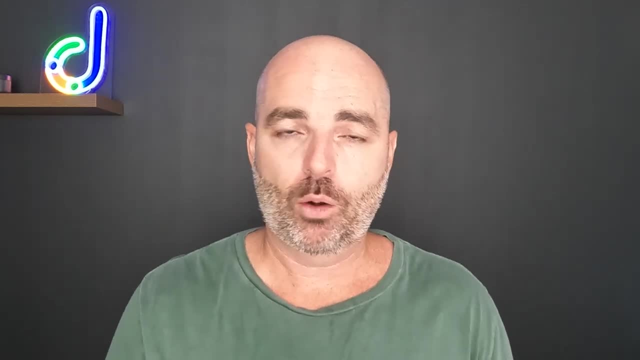 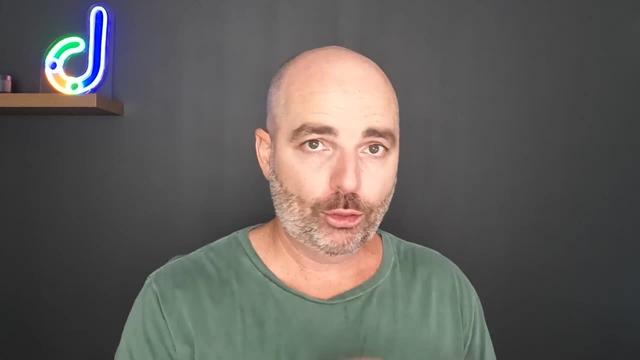 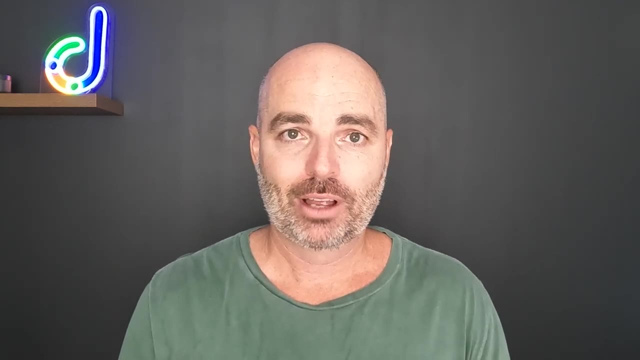 four different services go through into Google Ads. put those search terms into the keyword planner So you can look at that other data to find out which is going to be giving you a good balance of some keywords that do have traffic volume, because you need some traffic volume. 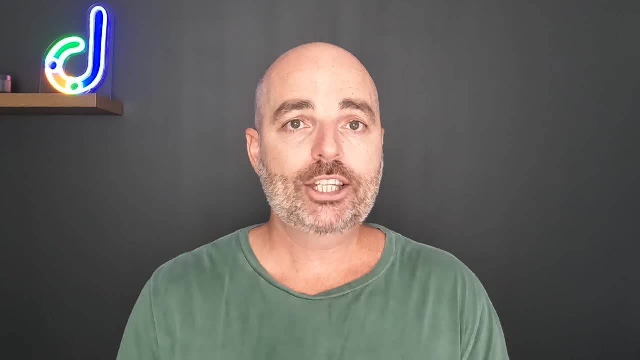 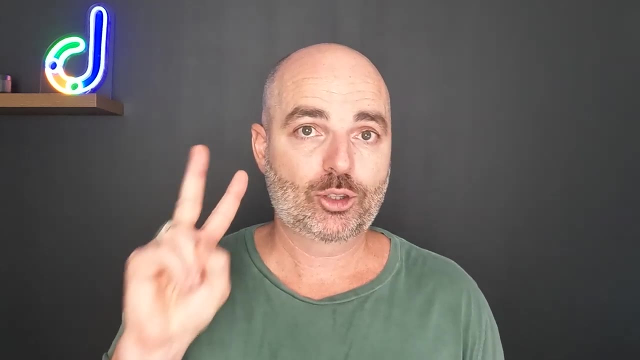 but that the cost per click is not going to be too high. So once you've gone through and, firstly, selected the best keyword themes and products to target for your business, that brings us to step number two And what we want to be doing here, especially for your search campaigns. 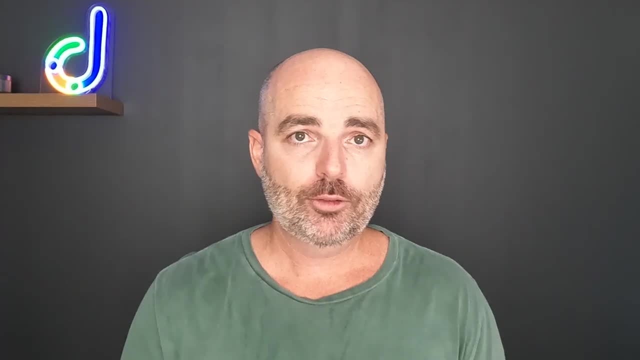 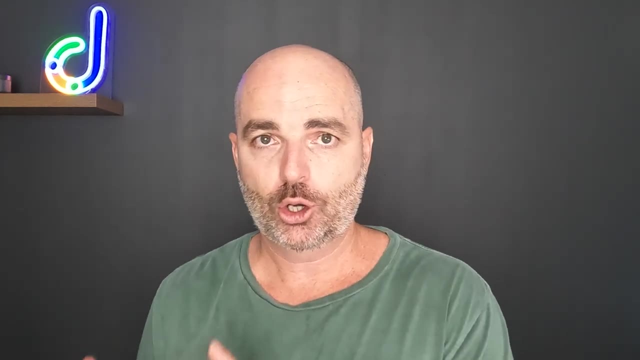 is: you want to be super aggressive with your ad copy. Now, the reason for why this is so important because, remember, in Google Ads you only pay for when someone clicks on your ad, not when someone sees your ad. So if you've got a small budget, what I like to do is use this to 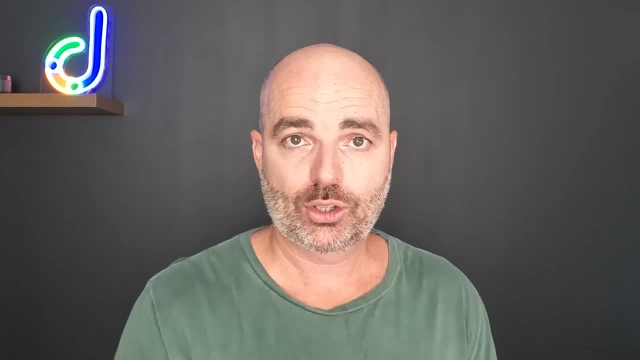 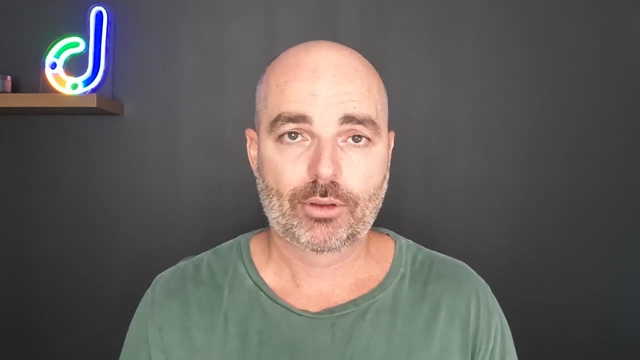 your advantage and start the pre qualifying process before they even get to your website. So what I mean by that is that in your ad copy you want to be super, super aggressive and start to filter people out so that if they see from your ad copy that your 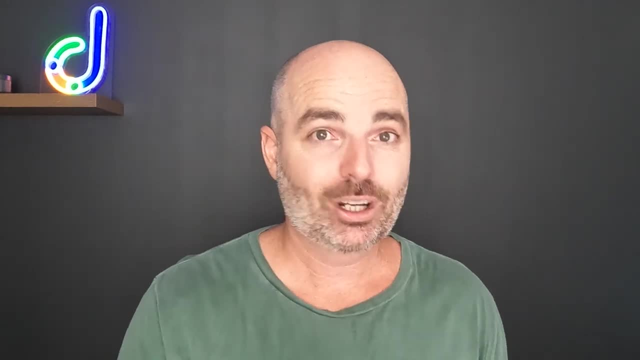 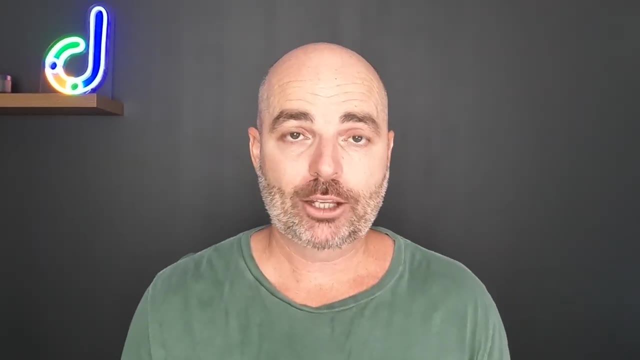 product or your service is not what they're looking for, they don't click on your ad because if you've got a small budget and they're not suitable, you don't want them clicking on your ad. So a great way to go about doing this is that I give really clear descriptions about what my 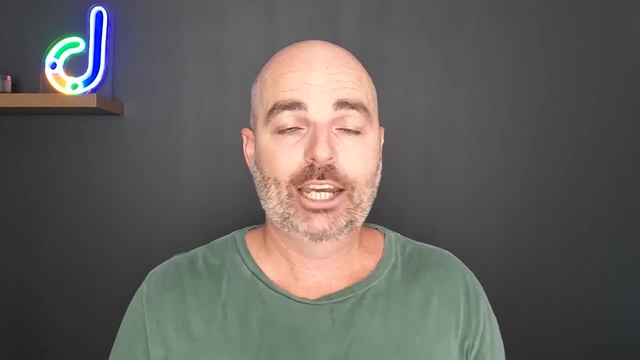 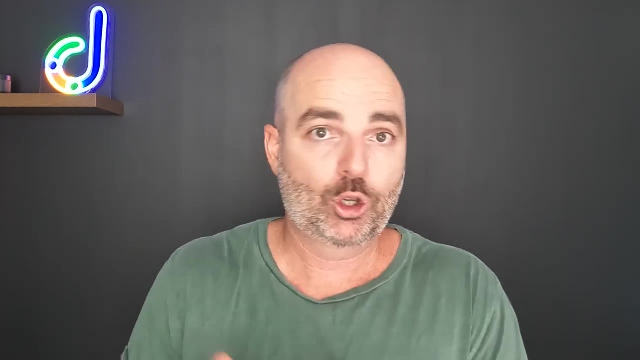 product or services are. If you're selling, say for example, t shirts, and you only sell shirts for certain age categories or certain sizes, you make it really, really clear that this clothes is suitable, say, for example, men over 40. Or if you've got a certain price. 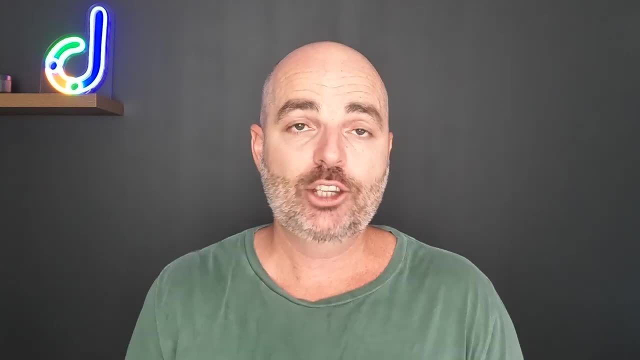 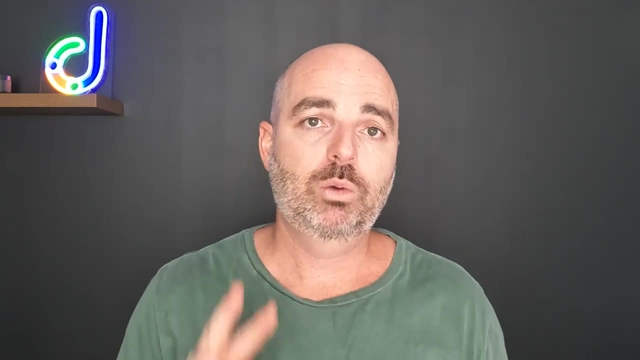 classification. So if your products are not the cheapest and you've got a higher price point than your competitors, I'd be putting your price in your ad copy. Now, yes, this will limit the number of clicks you have, But remember you've got a small budget, So you've got to fully capitalize. 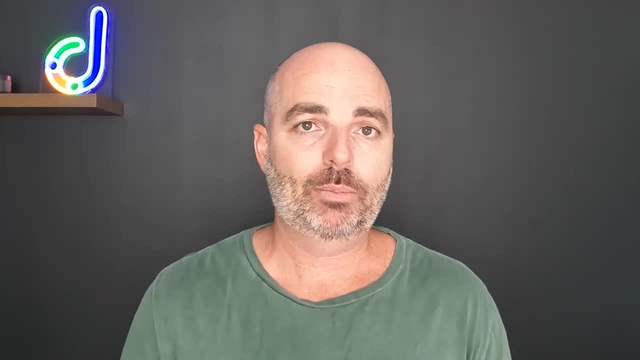 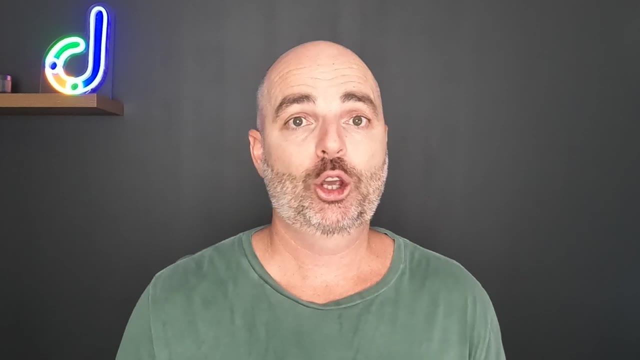 on every single click you get. So the next step is to be super, super aggressive in your ad copy and really use the ad copy as a chance to start filtering out and actually turning people away if they're not going to be suitable, Because- remember- 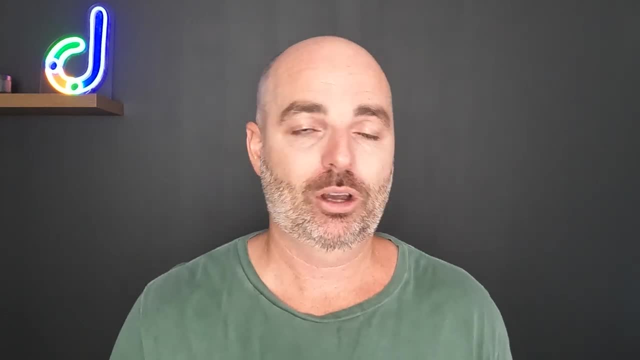 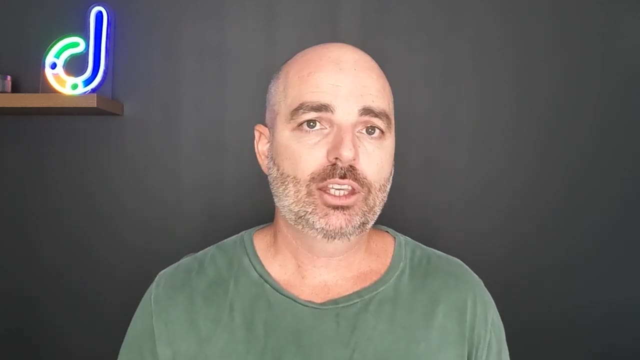 we don't want their click because we have to pay for their click if they're not going to convert. And then the third and final step in seeing success with Google ads, even if you've got a small budget, is that you need to be really realistic about your results that you can achieve in Google Ads. 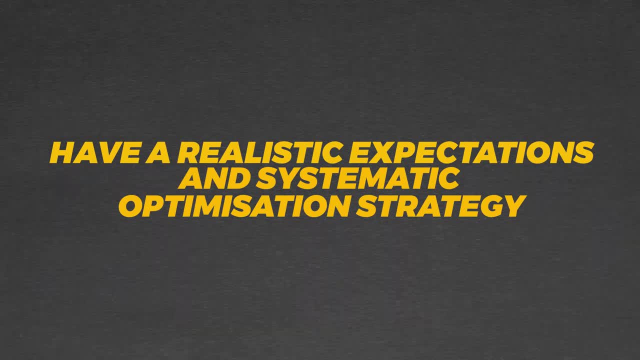 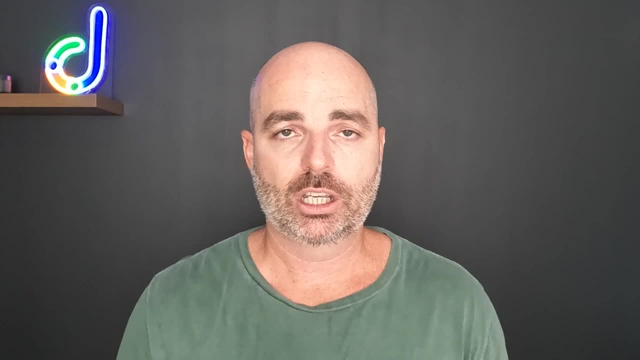 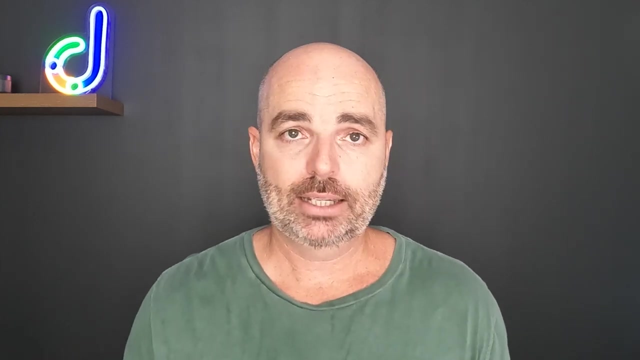 And you also need to have a systematic approach to optimizing. Now, I know that that is a really long point, But it is really really important. And the reason for why it's so important is because Google ads is a process And even if if you've got a high budget, it can still take 60 to 90 days before you're seeing the results that 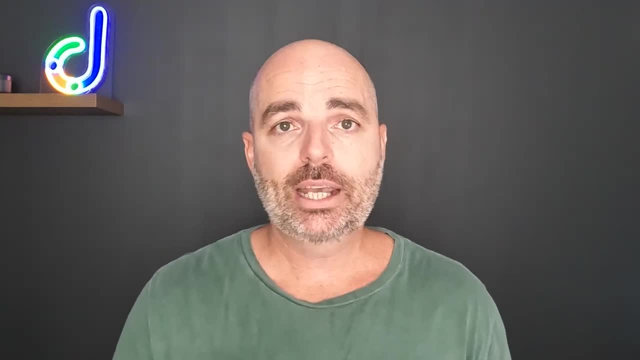 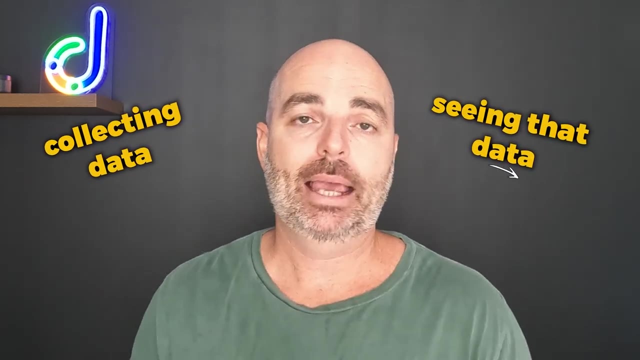 you need in order to break even or create revenue, And the reason for that is because success with Google ads is done through collecting the data, seeing that data and then making the relevant optimizations. And once again, remember- that's why I'm saying it's so important that you're 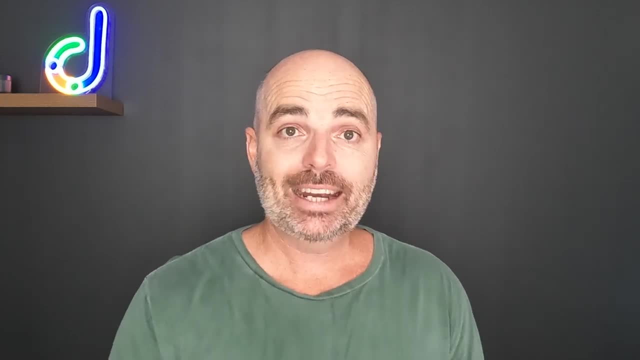 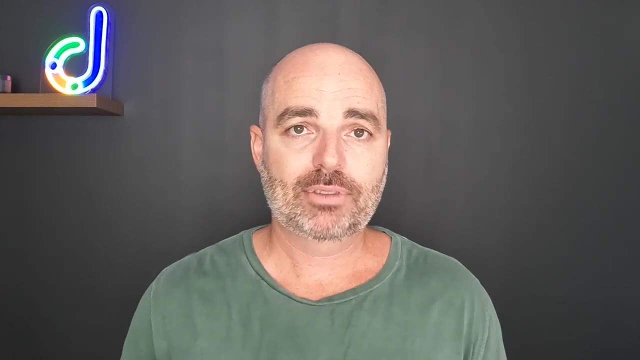 setting a budget that is at least getting 10 clicks a day, so that you've got enough data for you to be able to review, because if you run your ads for the first month and you've only got 10 clicks, you don't have enough data to be able to draw any real conclusions. So what I want to do 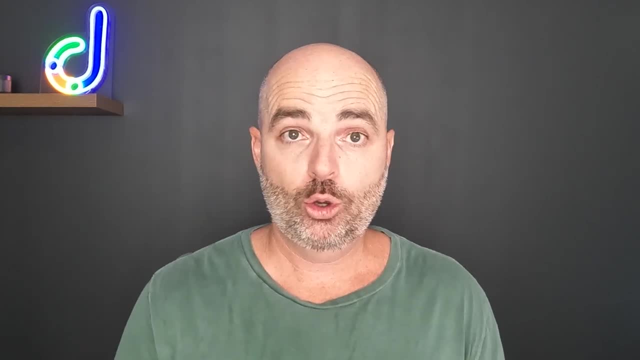 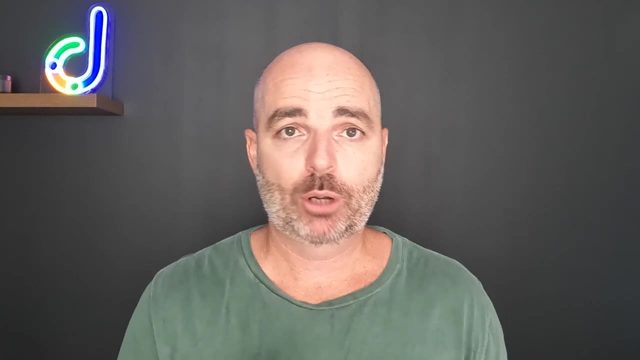 right now is we're going to jump into another screen share because I want to show you the lifecycle of a Google ads campaign over the first 90 days. But before we get to that lifecycle, I also want to give you access to my Google ads optimization checklist. And the reason for why. 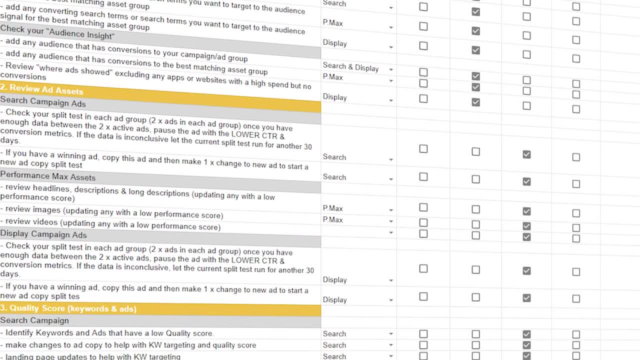 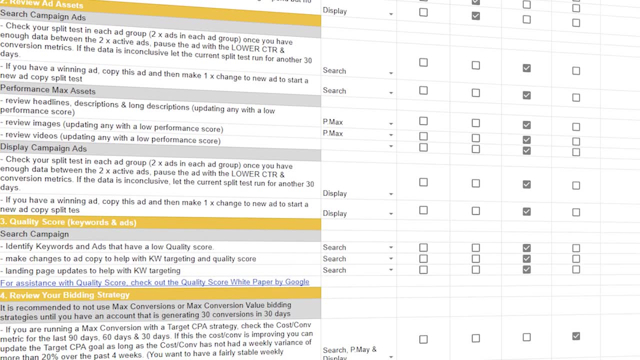 this is so important is: this is how you go through and systemize your optimizations, Because with Google ads, you can systemize your optimizations And you can systemize your optimizations And can over optimize your account, Because there's some optimization actions that you want to be. 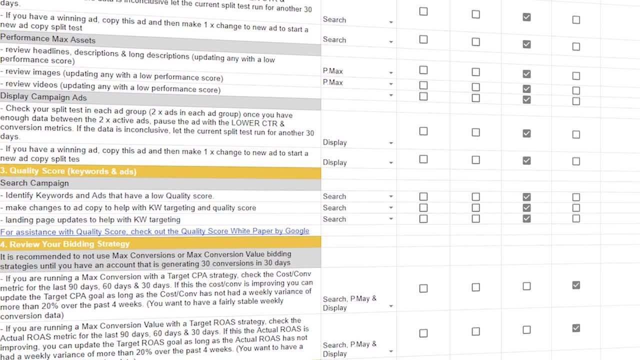 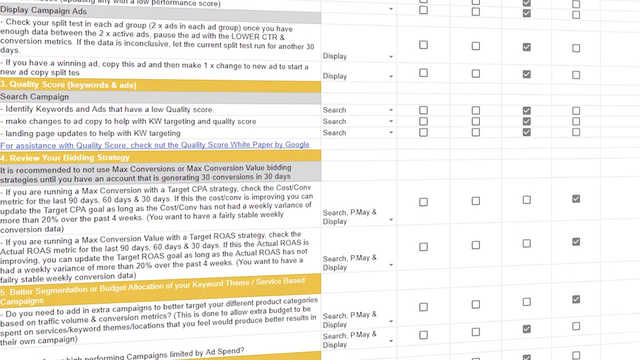 doing every week. there's others that you don't want to be doing until every month or every three months. The reason for that is because- remember what I said before- with Google ads, you want to be able to see the data, review the data and then make the optimizations. So if you want to get free, 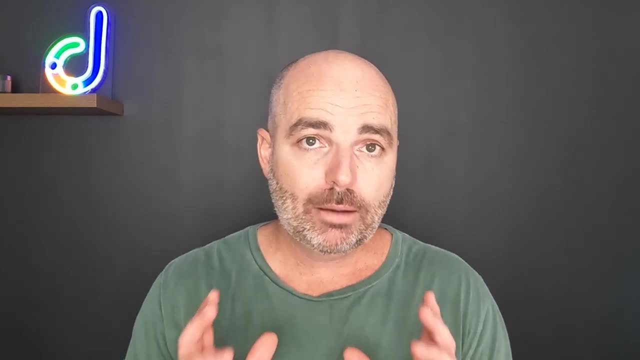 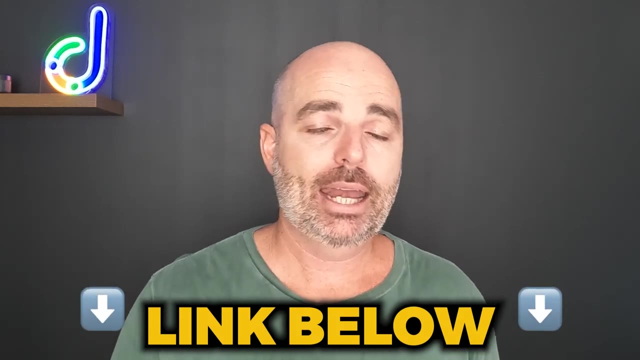 access to my Google ads optimization checklists so that you can best optimize your campaigns in 2024,. all you need to do is to follow that link in the description below And then, right now, let's go through and systemize your optimizations. 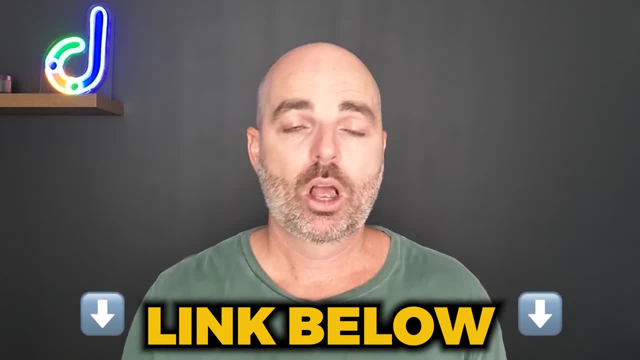 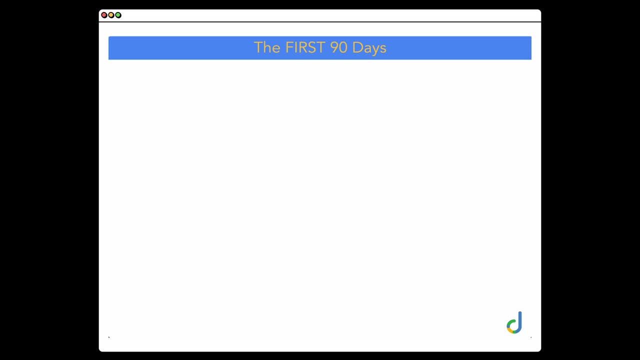 So I can show you the lifecycle of a Google ads campaign over the first 90 days. So what we've got here is the first 90 days of a Google ads campaign And I want to take you through the cycle that you'll be seeing- And this is really, really important, because this has always been the case- 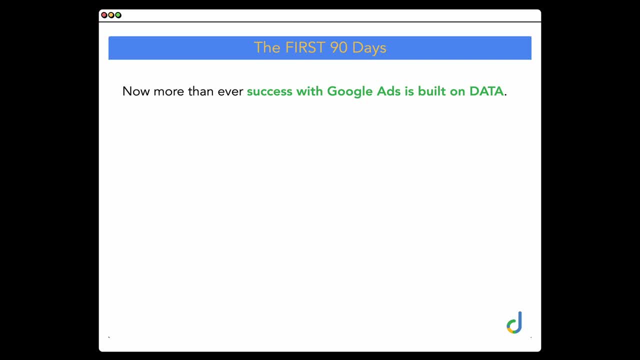 But now more than ever, success with Google ads is built on data. So what you want to be knowing that with any Google ads campaign, that you're running those first 14 days is very much a learning phase. Now we're not saying that you won't see conversions in that first 14 days And 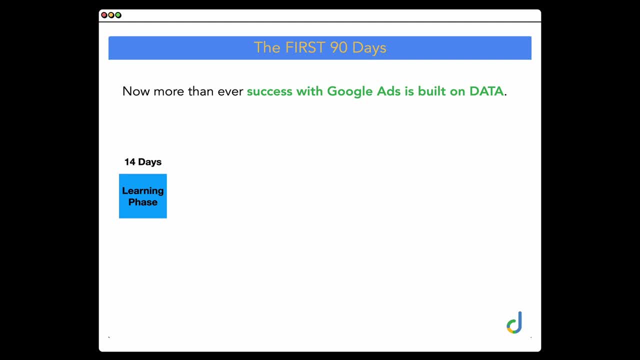 I have had some cases where you know we've turned the Google ads campaign on and within a matter of hours we're starting to get conversions already. But more often than not that first 14 days is just that initial learning phase. Don't be surprised if you start to see one day where 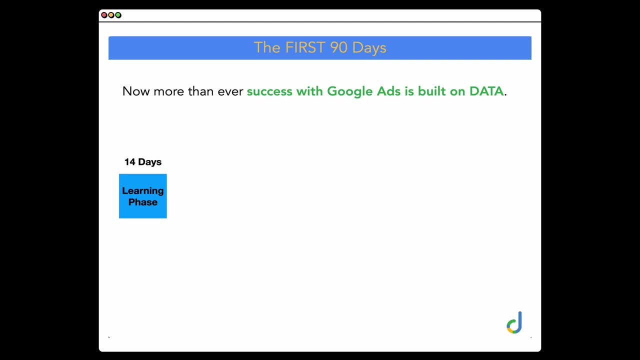 you'll see you know a good amount of clicks. you might get 10 clicks one day, then the next day you might get no clicks, And sometimes you may not get clicks for two days, And then you might come back with 15 clicks the next day. And this is all because Google is starting to run its own. 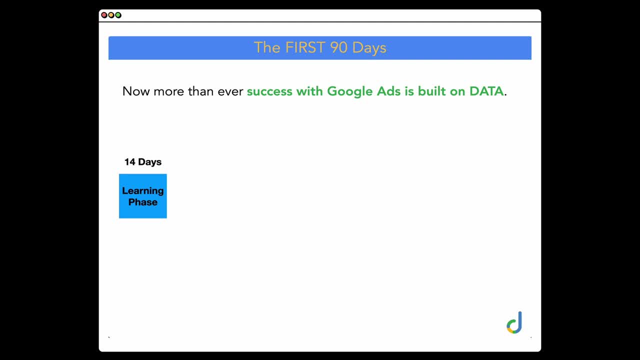 testing And it's comparing your ads versus your competitors, ads for your selected ads, keyword themes or products, And then what we want to wait to is after the first 30 days. this is the first time that we can really look through and get some initial data around our 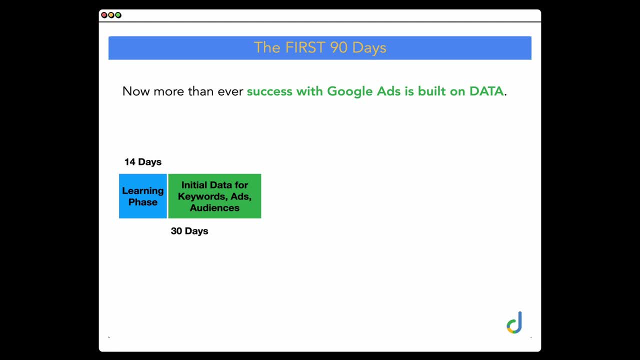 keywords, our ads and our audiences. And once you've got access to my Google ads optimization checklist, you'll see that inside this first 30 days, the only real optimizations that we are doing is we're going through for our search and shopping campaigns, reviewing our search terms. 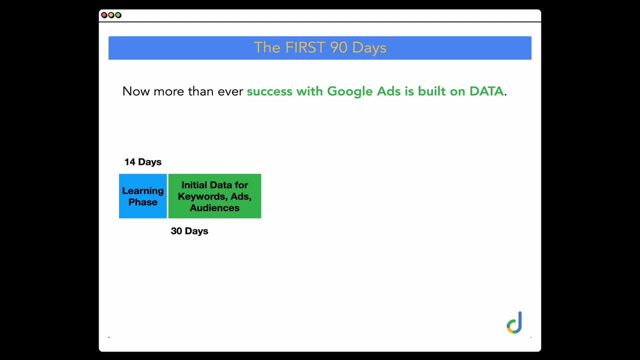 and adding in extra negative keywords. we can't run any split tests for ads yet, because we've got the split test set up, but we need to wait that 30 days until we get enough data, And that's when we then go through and start running some split tests. So then, what happens after the first? 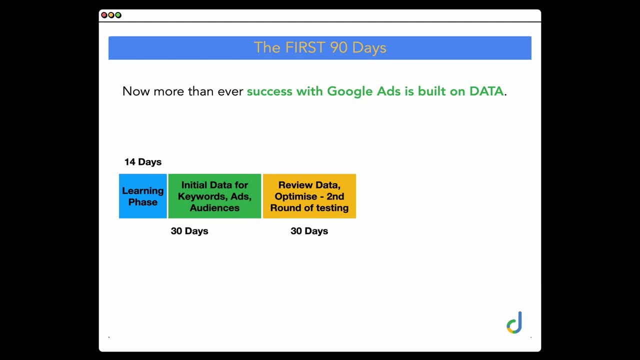 30 days is we review the data. we then optimize so we might add in some extra ad copy, split tests, And then from there we do a second round of testing And then from there we review the data, optimize and do a third round of testing. So you can see here- this is why sometimes you don't see. 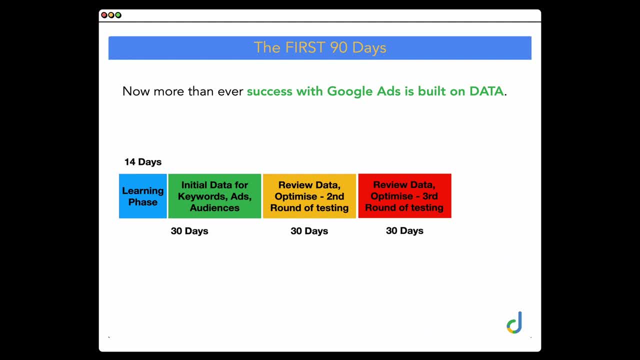 success for that first 90 days is because it may take us two rounds of optimizations and two rounds of testing Before we start to really get some breakthrough, And then from there we just continue to review the cycle. Now, as I said, in some cases you get success after the first 30 days, But more often 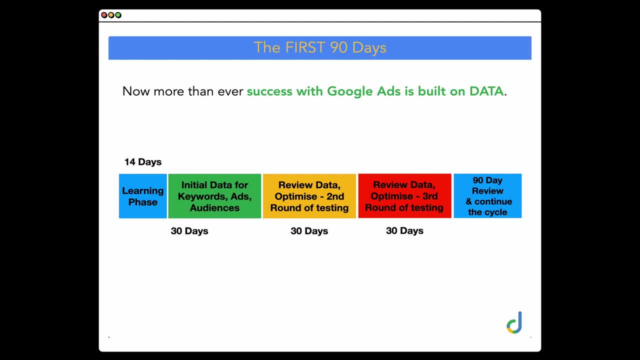 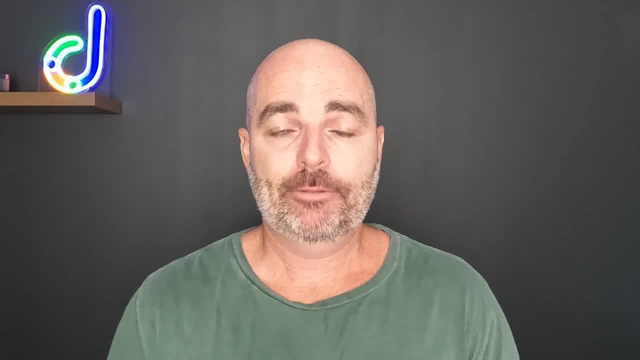 than not. it is taking this first 90 days until you start to see some significant results with Google ads. So finally, for Google ads, remember that you are giving Google ads enough time to be able to start to see some data so that you can go through and make those correct optimizations. 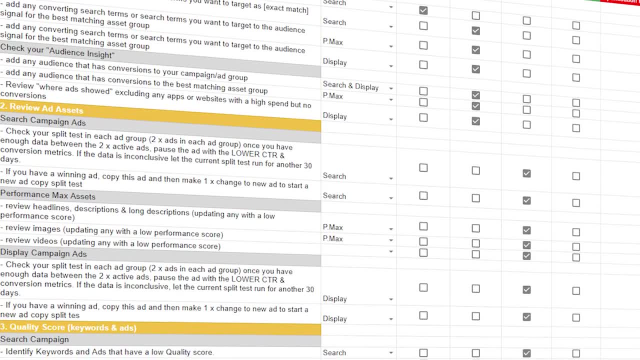 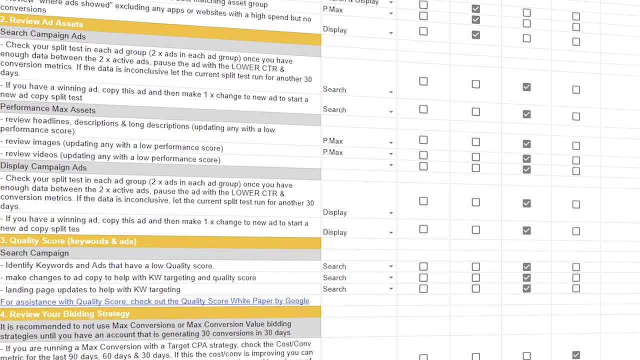 to your campaigns so you can see success And to help you with that process. remember to follow that link in the description below So you can get free access to my Google ads optimization checklists, which lets you know all of the different optimization actions that you need to. 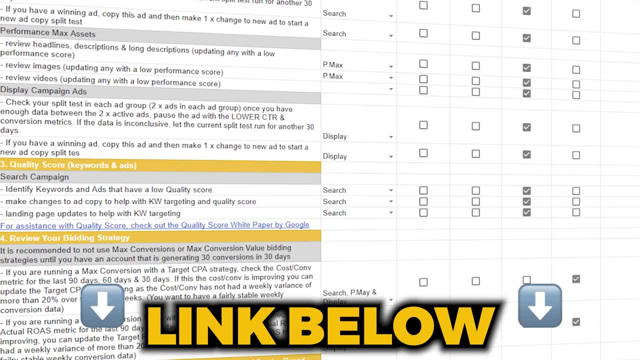 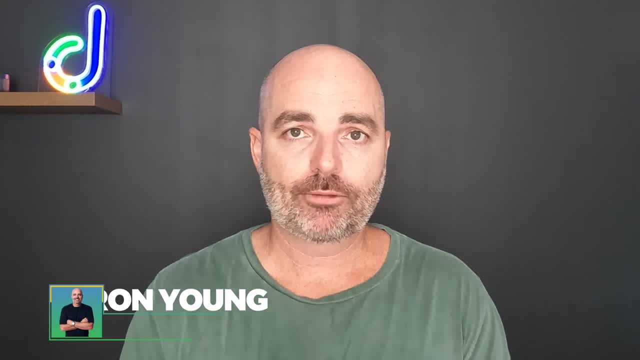 complete, And it also lets you know whether that action needs to be completed every 72 hours, every week, every month or every 90 days. Once again, thank you for joining me. My name is Aaron Young and I'm from Define Digital Academy, and I'm your 15,000 hour Google ads master, And it obviously